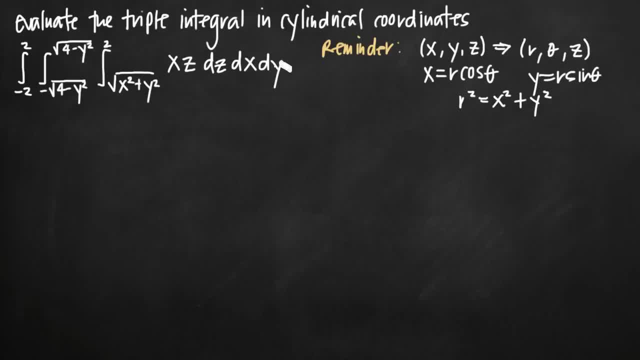 told that the order of integration is with respect to z, then x, then y, because we have this dz, dx, dy in this particular order, We need to convert this triple integral into cylindrical coordinates And, as a reminder, we have our standard Cartesian coordinates. 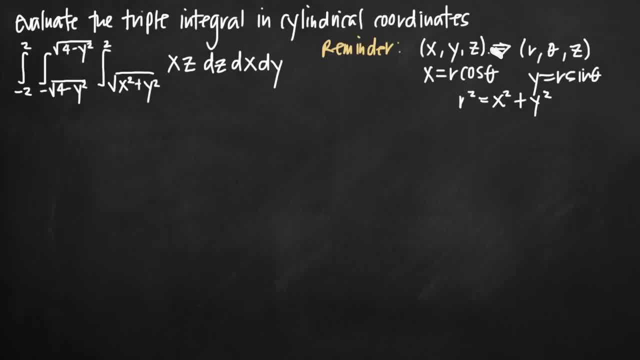 here x, y, z in three variables in three dimensions. When we convert that to cylindrical coordinates it looks an awful lot like polar coordinates. If you remember from polar coordinates when we were dealing with two dimensions or two variables in Cartesian coordinates, we had 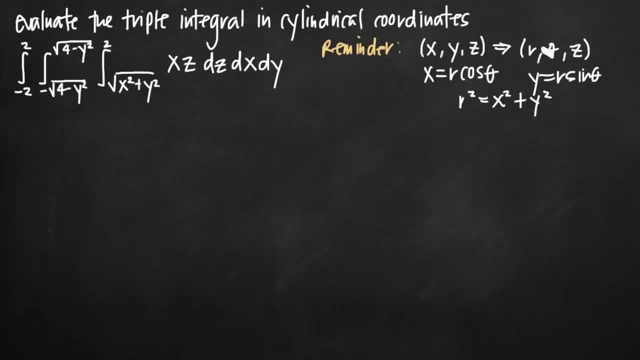 just x and y, And when we converted that to polar, we got r and theta. Well, you can see that with cylindrical coordinates we're going to do the same thing: X is going to become r, y is going to become z. So we're going to convert that to z And then we're going. 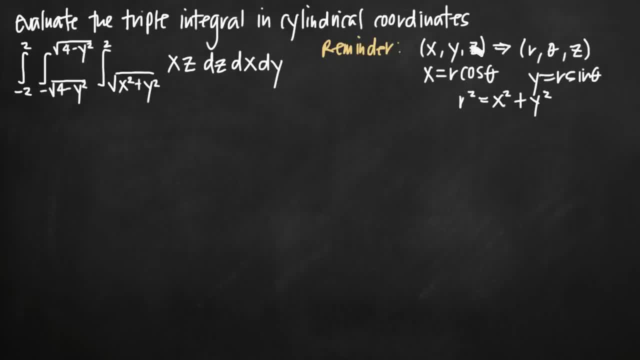 to convert that to r. y is going to become theta essentially, And z is going to stay the same here with cylindrical coordinates. When we add that third dimension to a Cartesian coordinate system, we also add it to the cylindrical coordinate system. It's going to stay the. 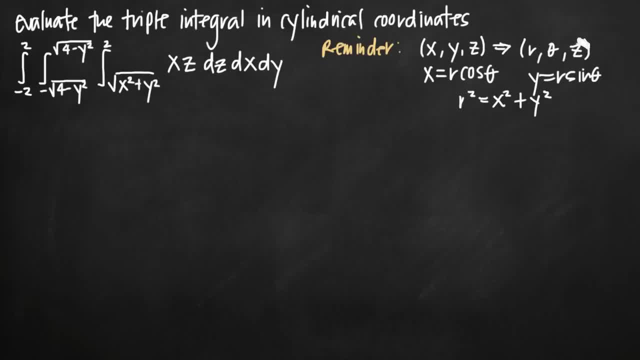 same. So z is going to stay the same across both coordinate systems. We're not really going to need to convert that variable. I've also got my conversion formulas for Cartesian coordinates to polar coordinates, If you remember. we have: x equals r times cosine theta, y equals. 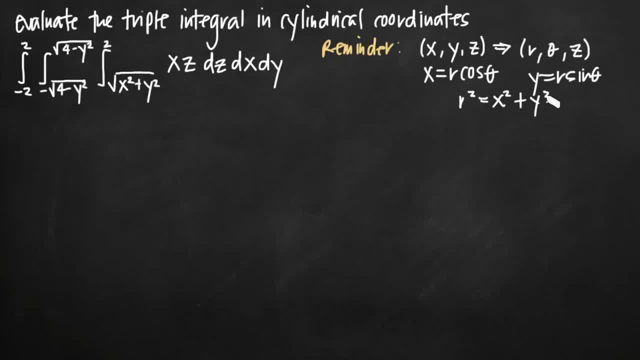 r times sine theta, and r squared equals x squared plus y squared. When we have a triple integral like this one that we're converting, we're going to need to convert three components: The function itself, which in our case is x times z. our order of integration, d, z. 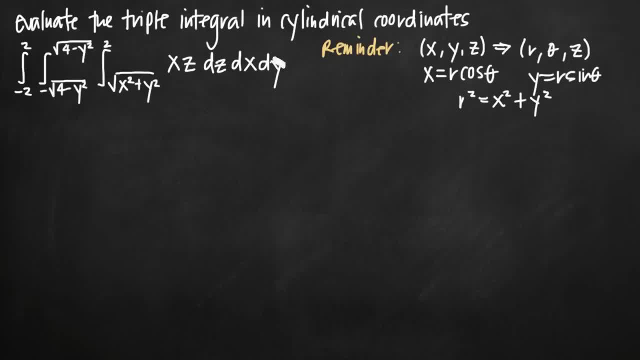 d, x and d? y is going to need to become d, z, d, r, d, theta and our limits of integration. So let's go ahead and start with our limits of integration so that we have those to write in. So our innermost limits of integration here are going to correspond with z, because z is. 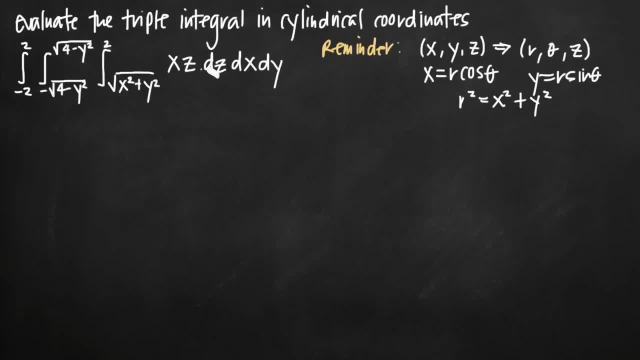 the innermost variable in our dz, dx, dy notation. here our order of integration. So we have z equals 2 and z equals square root of x squared plus y squared. Well, if you remember, we said that we didn't need to convert z because it stays the same. 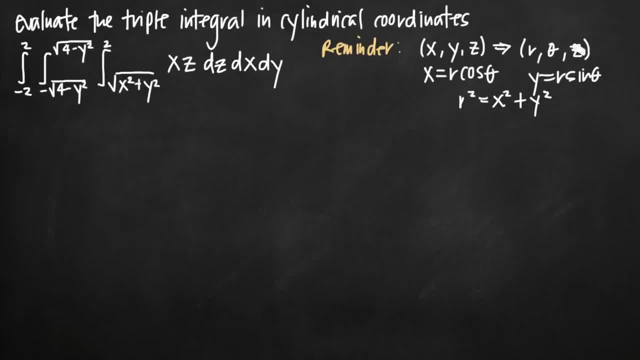 across two coordinate systems And for z equals 2, that's fine, because on the right hand side here of z equals 2, we have no x or y variables involved. but for z equals the square root of x squared plus y squared. we're going to need to change that x and y into r and theta. 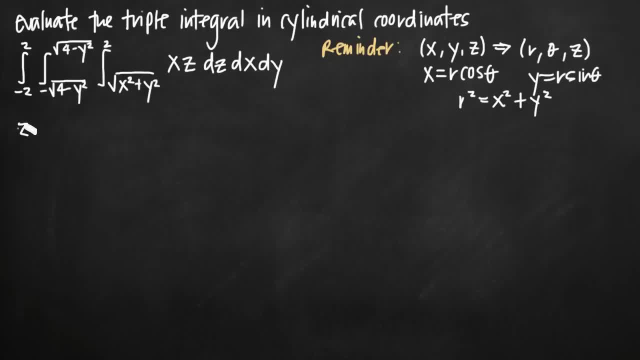 So we have z equals square root of x squared For x. we're going to substitute r cosine theta. When we substitute r cosine theta and then we square it according to that exponent. right there, we're going to get r squared cosine squared theta. 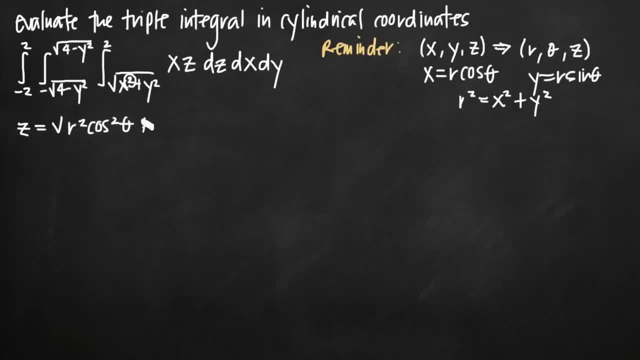 So we're going to have z equals square root of x squared. Then we're going to say plus, and here, when we plug in r sine theta for y and then square it, we're going to get r squared sine squared theta. This is our lower limit of integration, z. 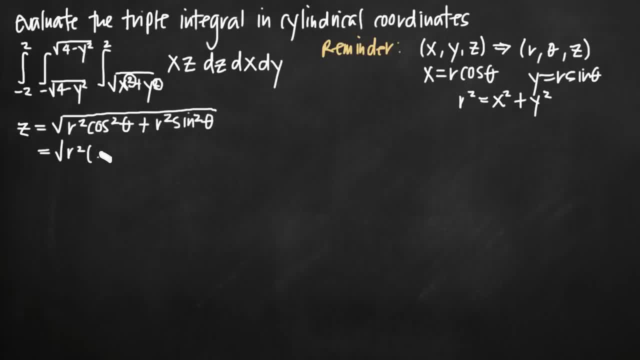 From here we can factor out an r squared, so we get r squared times cosine squared theta plus sine squared theta. And if you'll remember from our trigonometric identities, cosine squared theta plus sine squared theta is just the square root of x squared plus sine squared theta plus sine. 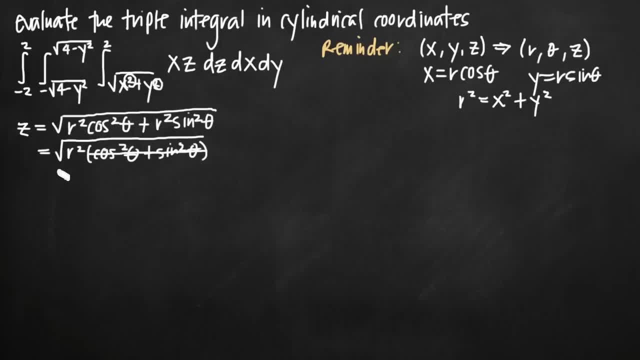 squared theta, So 1 and the square root of the square root of r squared, you get minus 1 and again you're going to get r squared Plus 1 is just equal to 1, so r squared times 1 is just r squared. 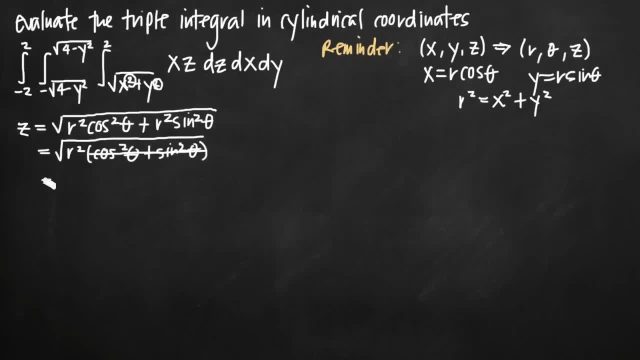 When we take the square root of r, squared, we're just going to get r, So r is our lower limit of integration. So our limits of integration for z, we'll write it up here. we'll say z is going to be from lower limit of integration r to upper limit of integration 2.. 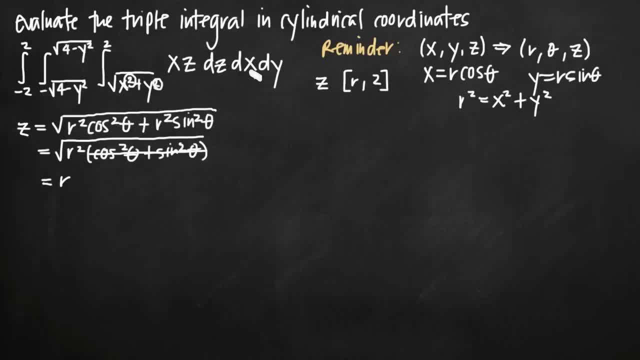 So we'll go ahead and write that there as a reminder. Now, our next variable here is x. We've got dx right to x, So we have essentially x equals the square root of 4 minus y squared. Well, if we make some substitutions, if instead of saying x equals, we say r, cosine, theta equals. 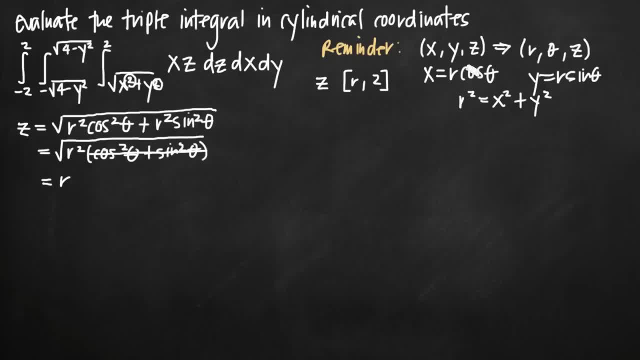 we use this conversion formula, we say r cosine theta is equal to. over. here on the right hand side we have square root of 4 minus y squared. so square root of 4 minus, but for y we're going to plug in r sine theta And when we square it according to that right, 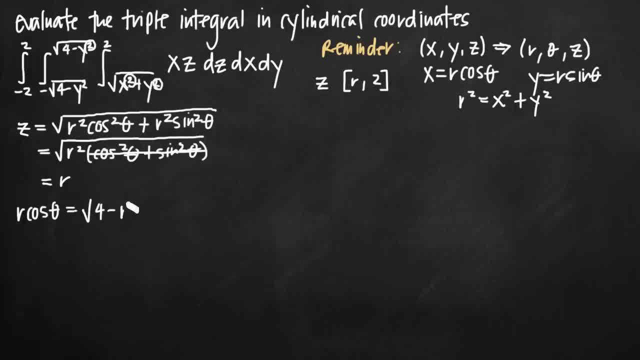 there we get r squared sine, squared theta. Now if we can just simplify this equation and solve it for r- because, remember, x becomes r over here- If we solve this for r, then we'll have our upper limit of integration for r. So what we want to do is square both. 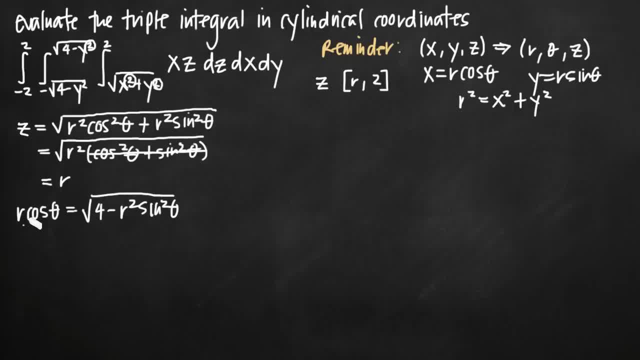 sides to get rid of the square root sign, We'll get r squared cosine squared theta and then we'll have our upper limit of integration for r. So we have: x squared theta is equal to 4 minus r squared sine squared theta, We'll add r. 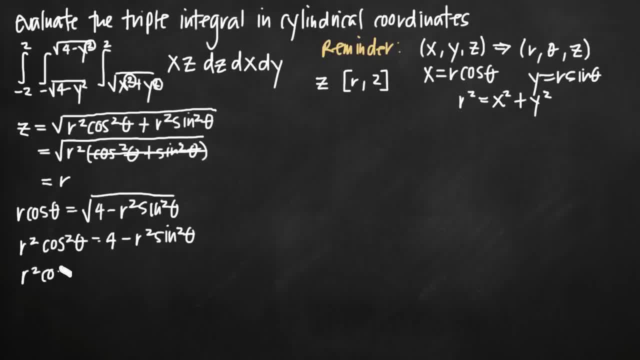 squared sine squared theta to both sides and get r? squared. cosine squared theta plus r? squared sine squared theta is equal to 4.. If we factor out an r? squared, we're left with cosine squared theta plus sine squared theta which, if you remember from this step, 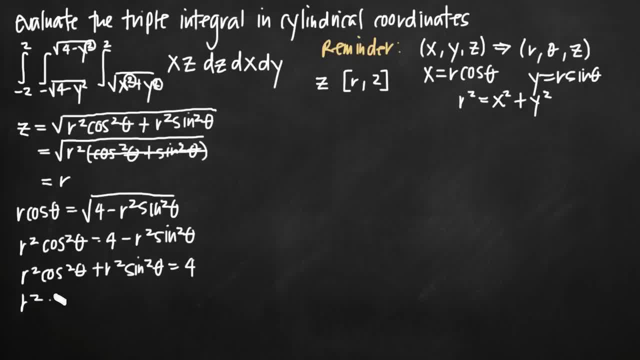 up here is just 1.. So we have r squared, sine squared, theta, Number zero and bottom 8 are 2.. And the minimum shotass is eyes in the distance. So now what you're going to do is, when we ask you, toishing is equal to 4, taking the 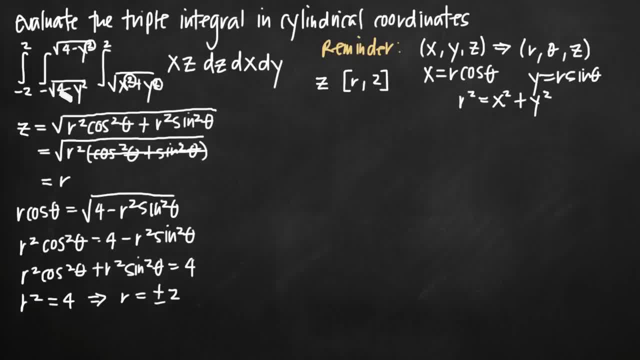 square root of both sides we get, r is equal to positive or negative 2.. Now if we did the same thing with this lower limit of integration for x and we said x equals negative square root of 4 minus y squared, and we plugged in our conversion formulas, 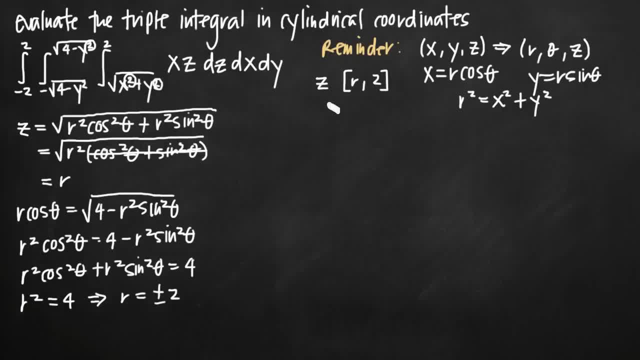 here we'd end up with the same answer: r equals positive or negative 2.. r- we're going to have r, negative 2 to positive 2, like this. Now, if we move on to y, we have dy here as our third variable. in our order of integration, That means our outermost integral. 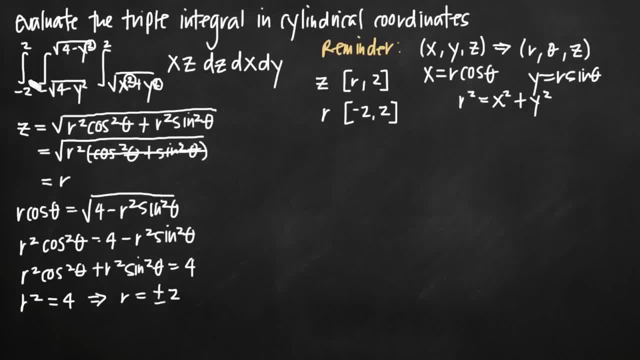 the limits of integration there relate to y. So we've got y from negative 2 to positive 2.. y is going to become theta. Well, theta is the easy one because, if you remember, the domain of theta is going to be from 0 to 2 pi, And that's going to be the domain of theta. 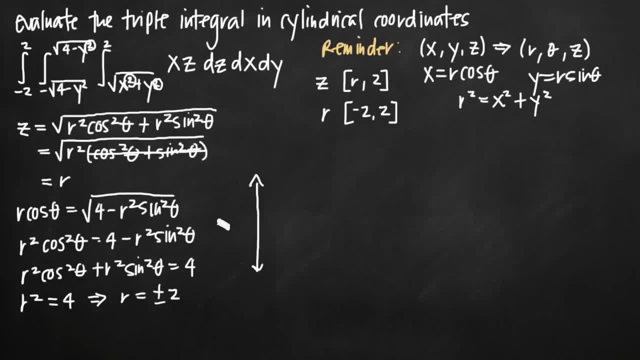 If we have our polar coordinate system here, if you remember polar coordinate system here and the angle starts at 0, goes all the way around here, our angle theta, until it comes back and at the point that it comes back it's 2 pi. So this is 0 and 2 pi The domain. 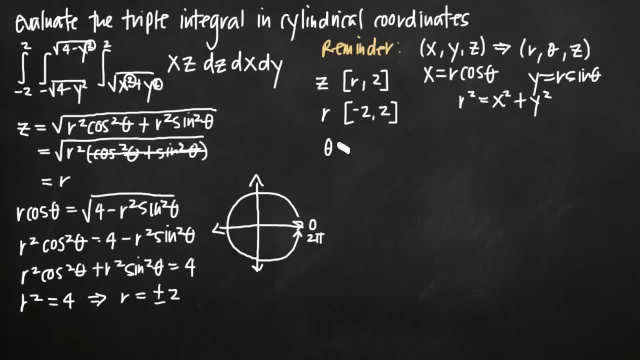 of theta, therefore, is just 0 to 2 pi. So theta is going to be 0 to 2 pi. We don't even have to use conversion formulas to find corresponding values for negative 2 pi. But what we can do is we can write out both problems. So we're going to do x equal to 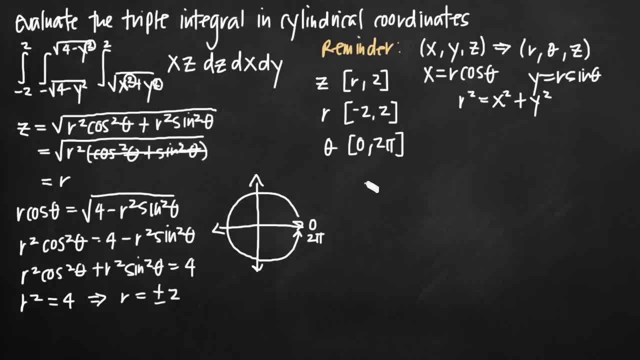 negative 2 and x equal to negative 2 and positive 2.. At this point we're almost ready to write out our triple integral. We can go ahead and start it and put in our limits of integration. So if we say the integral, we write our 3. 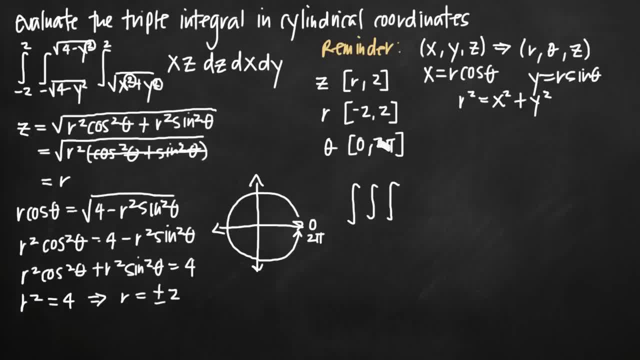 integrals here. We know that we're going to have our order here, dzdr d theta. So since d theta is last, we need our limits of integration for theta to come last. So 0 to 2 pi We're to be on the inside. so our innermost integral is going to be from r to 2.. Now, when it comes, 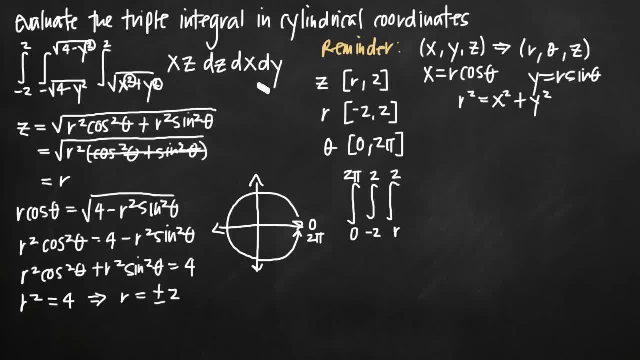 to our function x times z. z we leave alone because, remember, we say z stays the same across coordinate systems, but x we're going to substitute r, cosine theta. When we do this, when we convert from Cartesian coordinates to cylindrical coordinates, it's also very important to 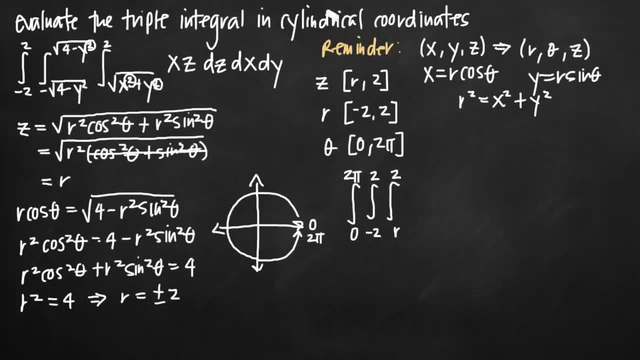 remember that whenever we do this, we need to go ahead and multiply by an integral of r. The coordinate systems don't translate perfectly in a direct way like this: x to r, y to theta and z to z, so we need to add an additional r. So normally for x we just 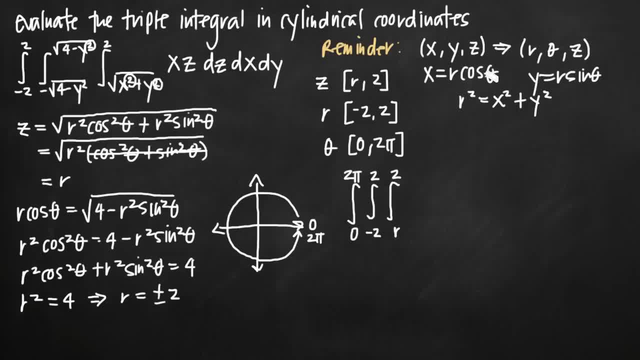 plug in r cosine theta, so we get r cosine theta. We multiply that by z. z stays the same, but we now need to multiply it by an extra r. We add an extra r. Your triple integral won't come out correctly if you don't multiply it by an extra r, So we need to add an extra. 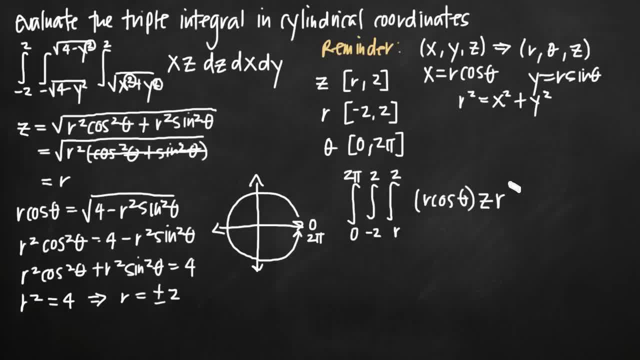 r, So we don't add this extra r in, So we've got r, and then dz dx dy just becomes dz dr d theta, And now, as you can see, we have no x's and no y's left over. We've completely. 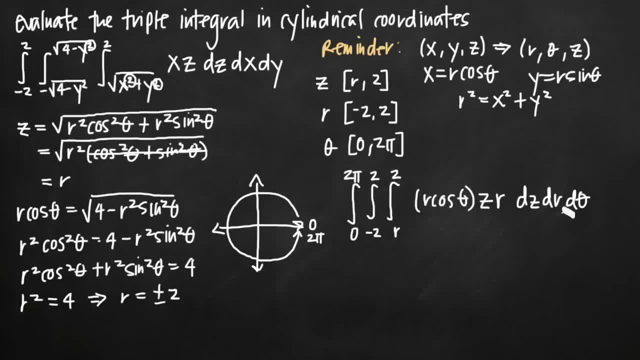 converted to cylindrical coordinates. At this point it's just a matter of evaluating this integral. So, because we have dz on the inside, we're going to integrate first with respect to z- We'll get the integral from 0 to 2 pi- and then we're going to integrate the 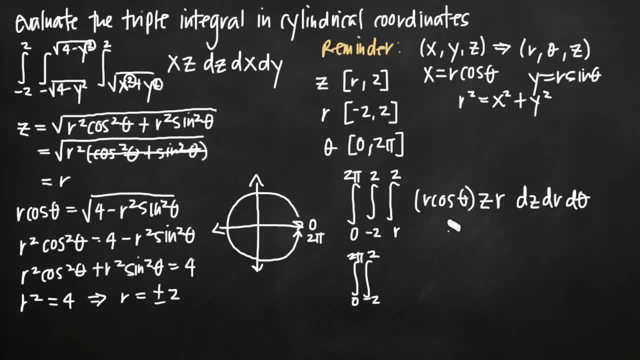 integral from 0 to 2 pi, the integral from negative 2 to positive 2.. And here integrating with respect to z. before we do that, let's go ahead and call this here r squared, because we have r times, r, z cosine theta. just to simplify it a little bit. 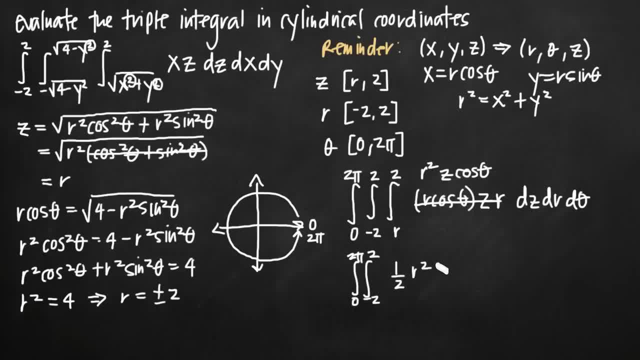 So, integrating with respect to z, we're going to get 1 half r squared, z squared. Remember, when we integrate with respect to z, we hold r and theta as constants, so they just stay as a constant coefficient on this z variable here. So they stay. We're going to be evaluating. 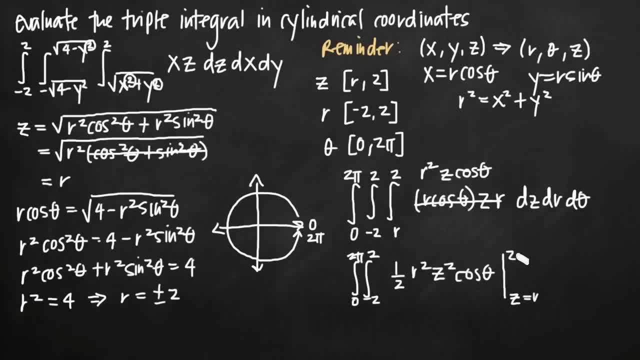 this on the interval z equals r to z equals 2, and we leave dr and d theta for later, Plugging in our upper limit of integration. z equals 2, we'll get 0 to 2, pi negative, 2 to positive, 2.. z equals 2, we're going to get 2 squared, which is 4.. Dividing that by: 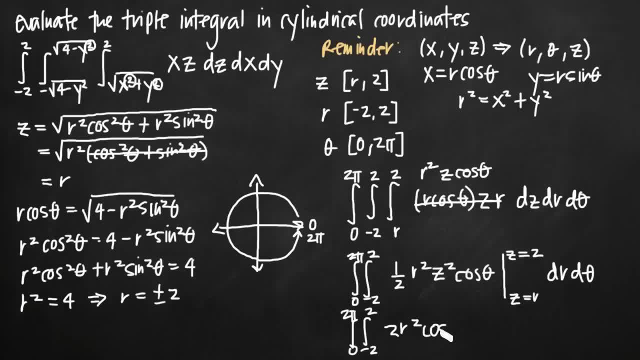 2, we're going to get 2 pi, So we're going to get 0 to 2 pi, So we're going to get 2 r squared cosine theta and then, subtracting whatever we get, when we plug in z equals r, we get minus 1 half r squared times. plugging in r for z r squared again gives us r to. 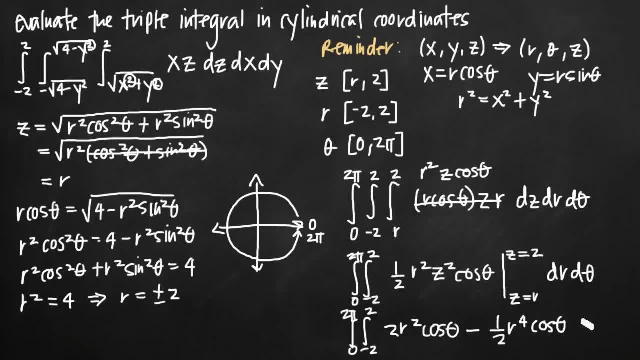 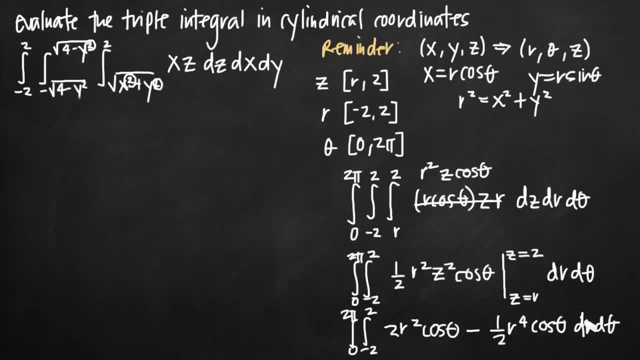 the fourth, and then cosine theta, dr d theta. Now, according to our order of integration here, our next integration variable is going to be r. We're going to integrate with respect to r, So we're going to leave 0 to 2 pi out. 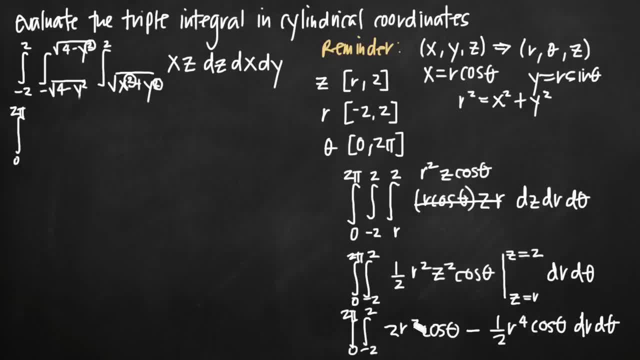 here for theta And then integrating with respect to r, we're going to get 2 thirds r cubed cosine theta. Then we're going to get r to the fifth, but we got to divide by 5, which means we're going to get minus 1 tenth r to the fifth cosine of theta And we evaluate that on the interval. 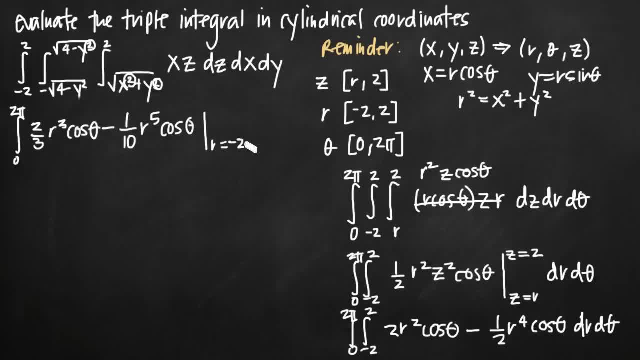 r equals negative 2 to r equals positive 2, leaving d theta out here for later, Plugging in our upper limit of integration. we're going to integrate with respect to r and we're going to get r to the fifth and we're going to get for our upper limit of. 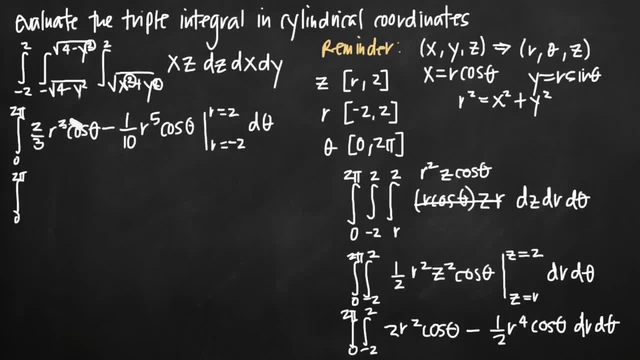 integration r equals positive 2.. 2 cubed is 8 times 2 thirds is 16 thirds cosine theta. minus r to the fifth is 32. so we get minus 32 tenths cosine theta. Now we're going to subtract whatever we get when we plug in negative 2, so minus here. 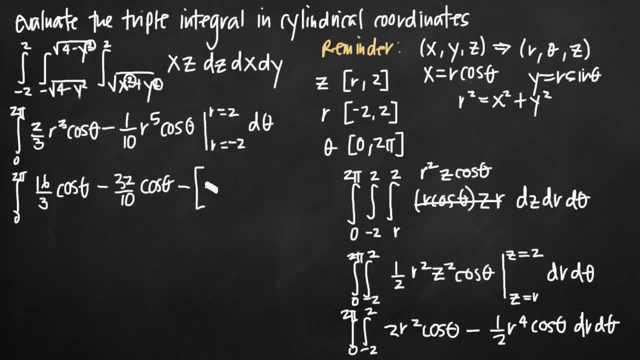 Negative 2: cubed is negative 8.. So we're going to get a negative 6.. cosine theta. Negative 2 to the 5th is negative 32. so we're going to get negative 32 over 10. but we have this negative sign, so we're going to get plus 32 over 10. cosine theta. 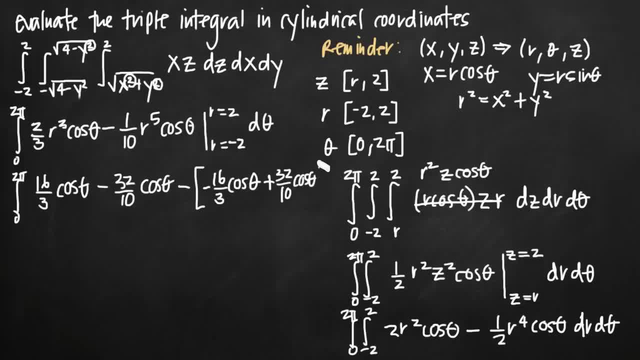 and then we'll leave our d theta out here for later. We need to do some simplification here. We're going to end up with 16 thirds cosine theta minus 32 over 10 cosine theta minus a negative. 16 thirds is positive, 16 thirds cosine theta and then minus a positive. 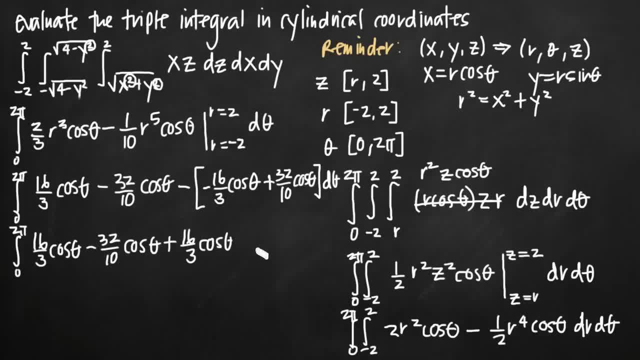 30 to 10 gives us just a negative 32 tenths cosine theta d theta. Now we can combine all of these and we can get negative 32 over 10 cosine theta. So this is our d theta denominator is 30. So in order to get a common denominator of 30 and all this stuff to get 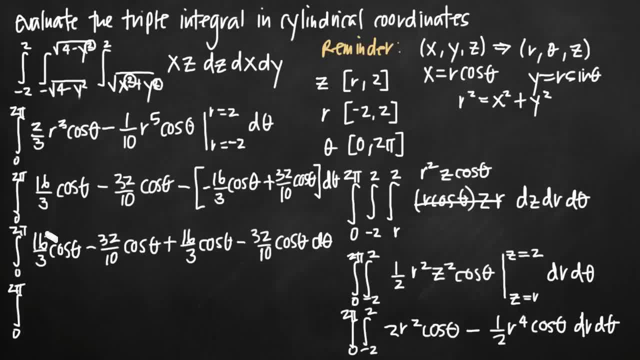 16 thirds. we'll multiply by 10 over 10.. That's going to give us 160 over 30. cosine theta Here for 32 over 10, we'll multiply by 3 over 3.. That's going to give us minus 96 over 30. 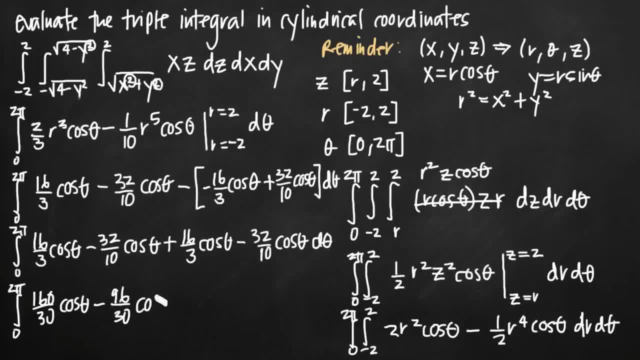 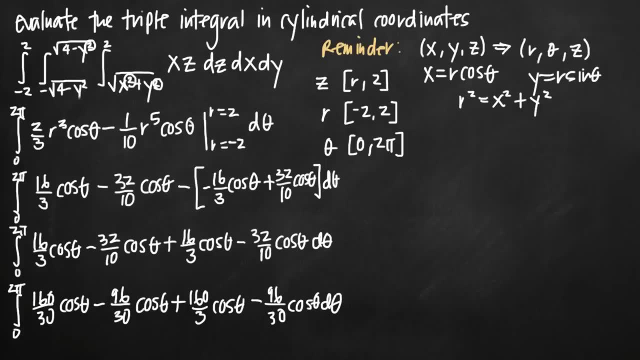 cosine theta plus 160 over 3 cosine theta minus 96 over 30 cosine theta d theta. If we do the arithmetic there and then reduce our fraction, we're going to end up with the integral from 0 to 2pi of 64 over 15 cosine theta minus 96 over 30 cosine theta minus. 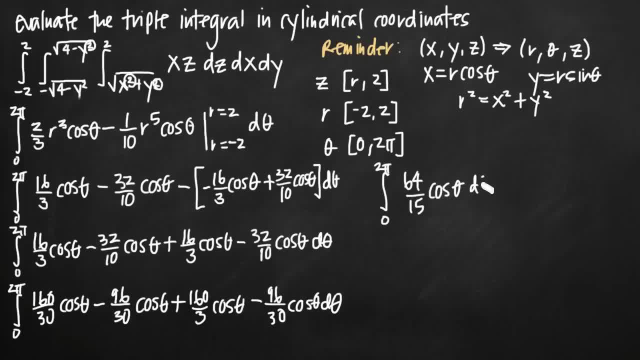 96 over 30 cosine theta. with respect to theta we're going to get 64 over 15 times sine of theta. but then we need to evaluate that on the interval theta equals 0 to theta equals 2 pi Plugging in.